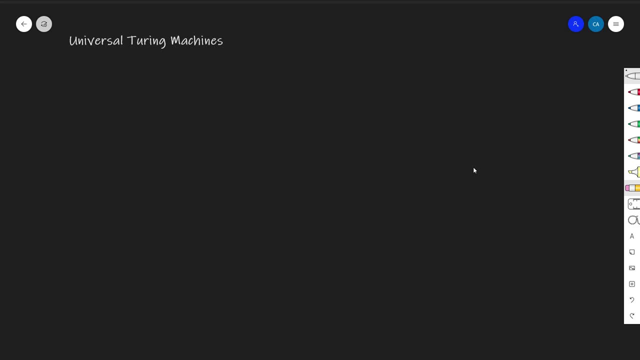 Because once I start doing examples of it, you're going to start feeling a lot weirder about it, I think, than you do currently. So what I'm going to do to condition you for that is that we're going to have one very short video where I explain to you what a universal Turing machine is. 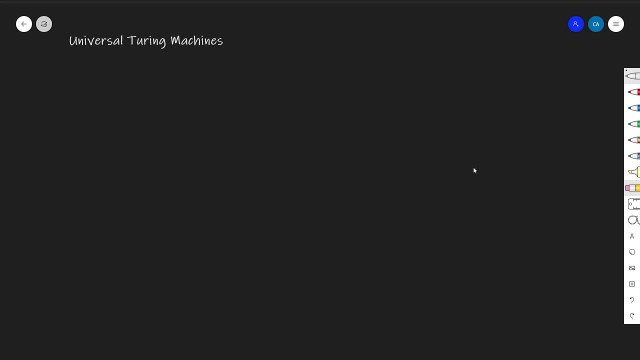 And I show you why. a universal Turing machine has to exist by the Church-Turing thesis. And this video is going to be very short and you're going to walk away from it feeling utterly unsatisfied, Okay, But nonetheless completely convinced. 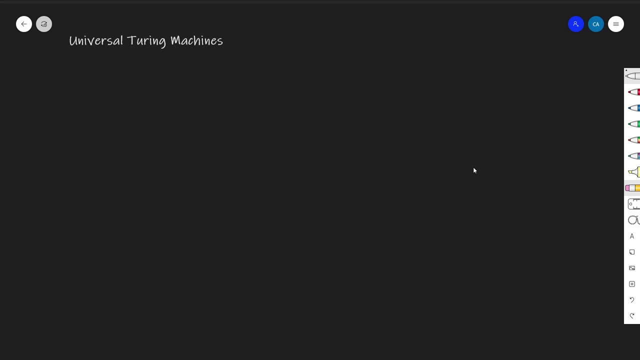 So let's get started on that. So what is a universal Turing machine? Well, a universal Turing machine is, in a sense, more of a computer than you're used to in terms of what we've been talking about. So what we've been talking about so far are machines that do specific tasks, right? 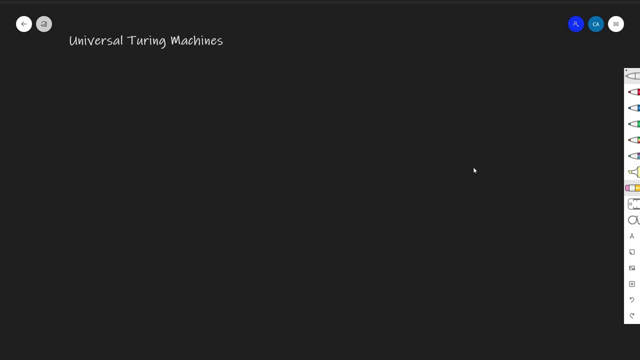 I talk about a Turing machine that adds numbers, or a Turing machine that detects palindromes or figures out if a number is factorable. right, They do specific things. But what your computer does, the one that you're using to watch this is, it does well anything, right. 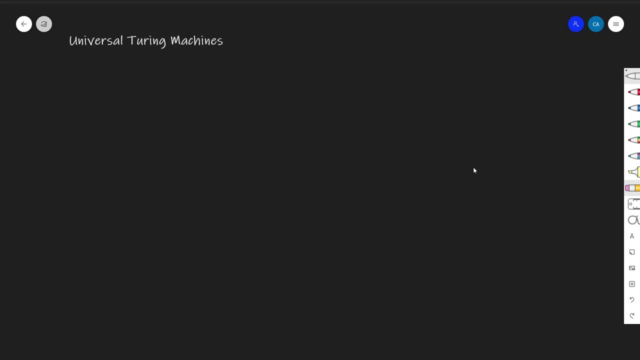 It does what you tell it to. And how do you tell a computer to do something? Well, you feed it a program, You feed it a string of text and then it processes that text and it basically simulates another machine. So your computer is a universal Turing machine. 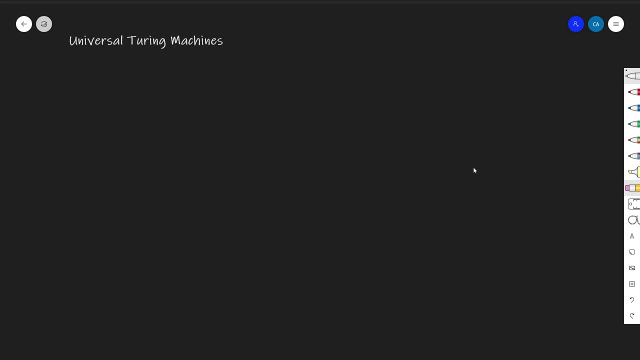 It takes as input basically other machines, and then it simulates those machines in the way that you want them to, And so that's exactly what it is, But let's define it in terms of Turing machines, So a universal Turing machine, which will often denote UTM. 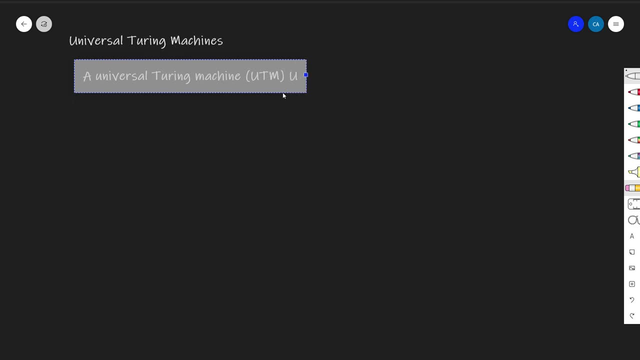 and we'll call it as a machine. U is a Turing machine which takes as input two inputs. right, It takes in two inputs: One, it takes another Turing machine which will denote M, and then two an input to that Turing machine. 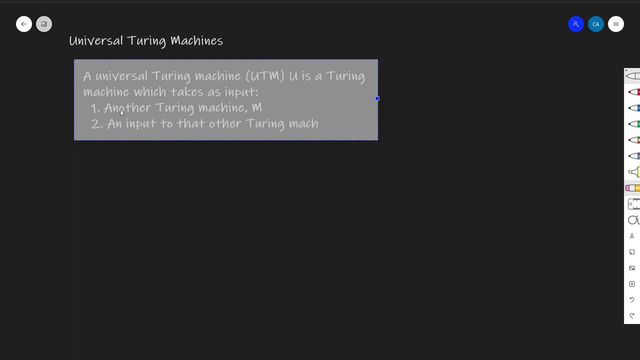 that other Turing machine x and which returns as output M of x. So basically, the UTM as a machine U takes as input a machine M and an input x, and then it spits out M of x. And that's exactly what your computer is doing right now. 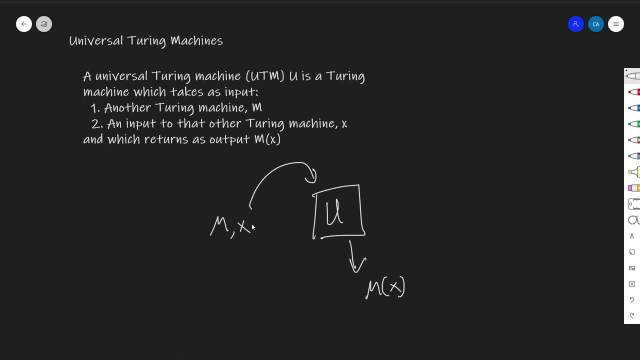 It's taking as input other programs and then input to those programs. For example, you use Microsoft Word and you type things into it. You're giving that program input and then your overall machine, your universe of the machine, your operating system. essentially, 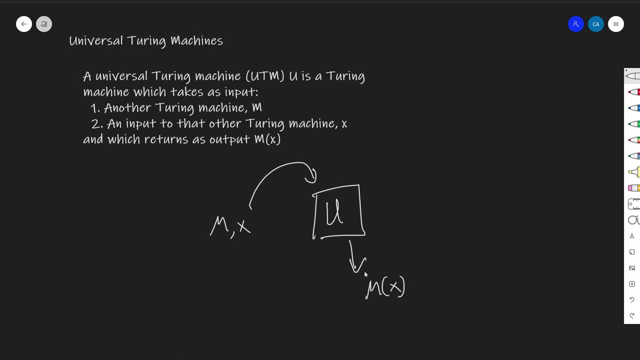 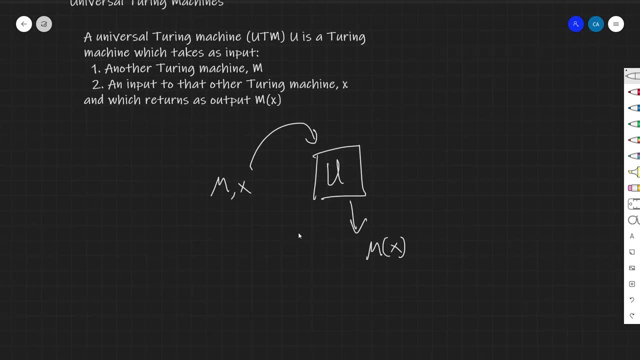 is producing M of x continuously, And that's exactly what a universal Turing machine does. So- and by the way, this might look strange, Another Turing machine as input. How does that work? Well, remember, just like your programs, that you write. 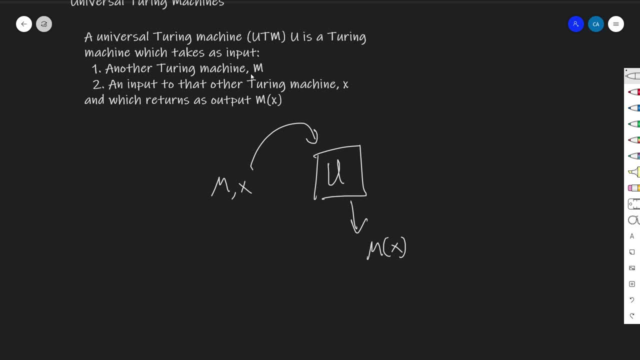 when you write a program and you have it run, that's a finite program. You write essentially essentially any program you write in Java or C++ or whatever. that is essentially a finite string. And we noted that Turing machines, you could write them down on paper. 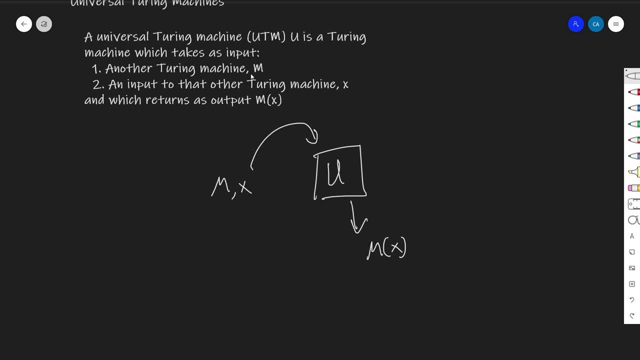 just like that. If you recall the addition- the Turing machine we designed that performs addition- we just kind of wrote the instructions down one at a time, And we noted that you only need to write down a finite number of them, And so Turing machines are finite strings. 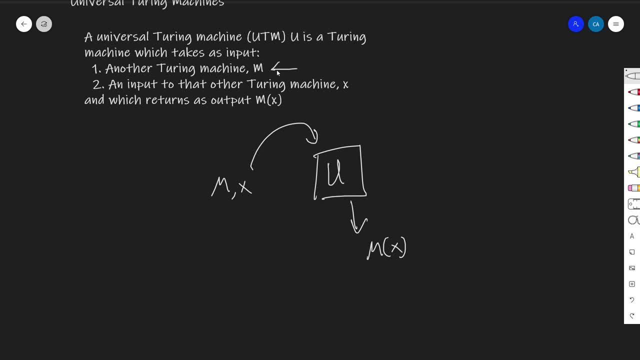 You can code them easily, naturally, as finite strings, Because I can write down- not because, but you know, I can write down- a string, little m, I'll call it, which syntactically specifies m, capital M. 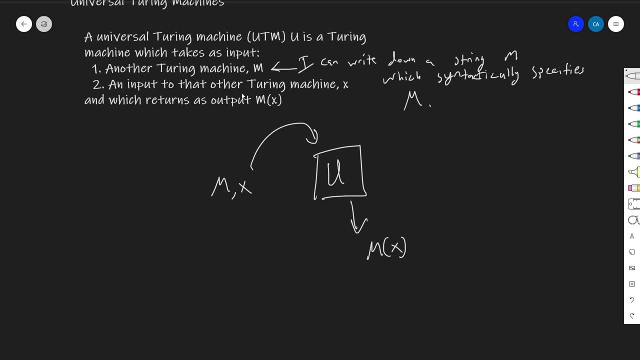 So I can write a string down that describes n, because I can give you m on paper. If I could do an example for you right now, I could say: design a Turing machine that does this, and you could write down the Turing machine as a finite string. 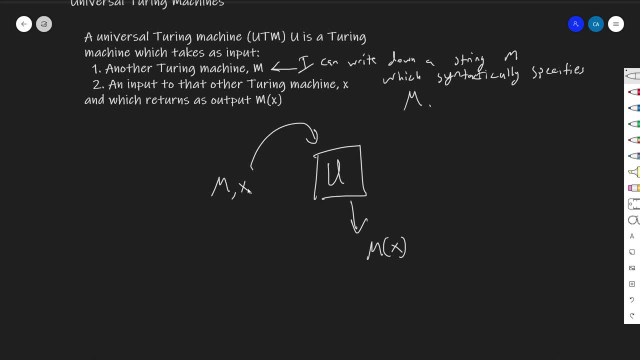 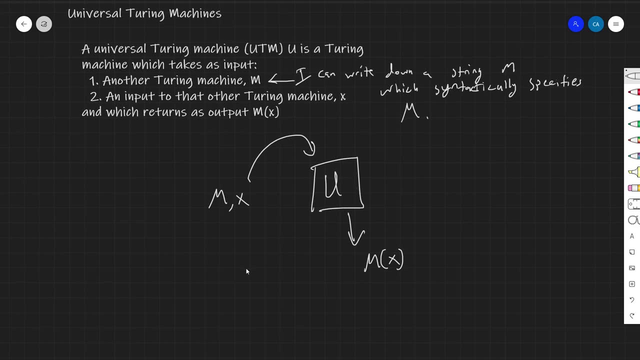 And so that's exactly what this machine U takes. It takes that finite string that gives you the Turing machine on paper and then an input to that Turing machine and it spits out the output. So hopefully that makes sense. That's what a universal Turing machine is. 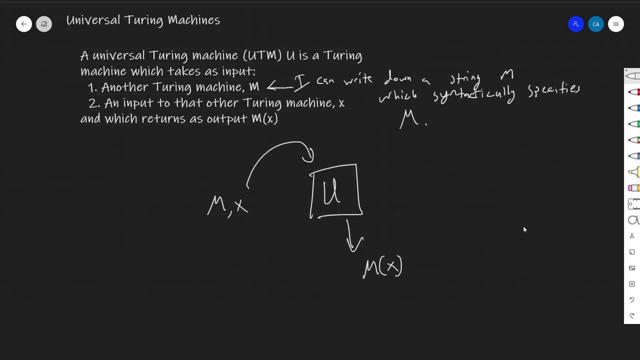 and we're going to make extensive use of it. We need to have noted that it exists in order to kind of continue what we're doing. And so what we want to ask with this video is: why does it exist? So does such a Turing machine exist? 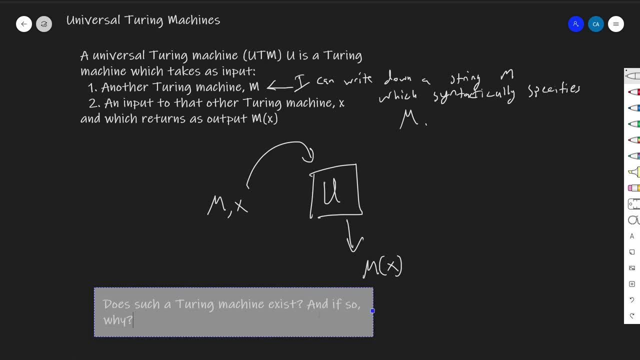 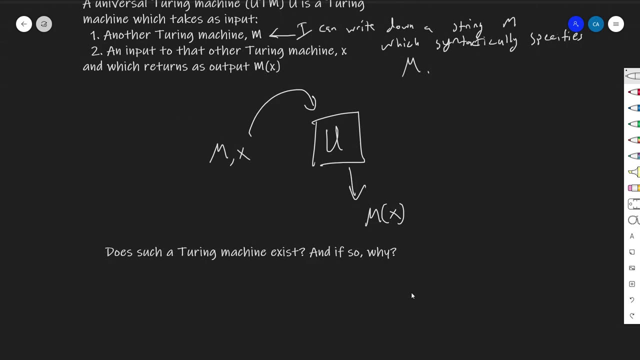 And if so, why So? if this was a real, if this was a rigorous thing, if this was like rigorous math, then what I would have to do is design one for you, like actually explain how it works. But we don't really need to do that. 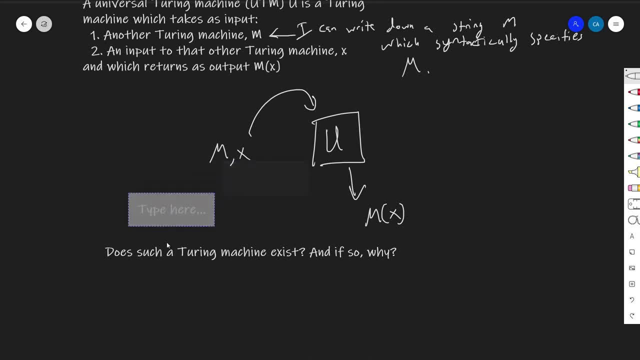 because check out this argument, this thoroughly unsatisfying but also thoroughly convincing argument. Thoroughly convincing, assuming you understand the Turing thesis- So you might walk away from this video and you might have to do some thinking about it, but that's why I'm making it intentionally short. 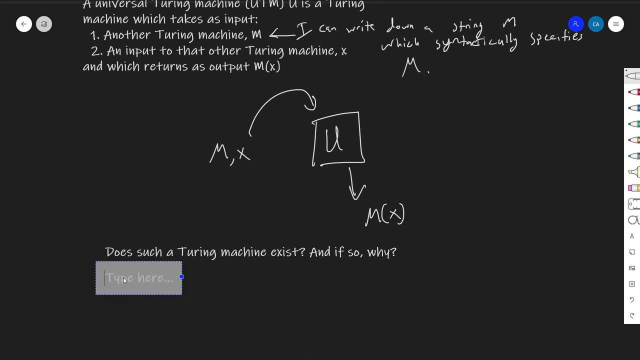 kind of to frustrate you a little bit. So here's why a Turing machine, here's why such a, here's why a universal Turing machine exists. If I gave you on paper a description of a Turing machine M, we'll call it M. 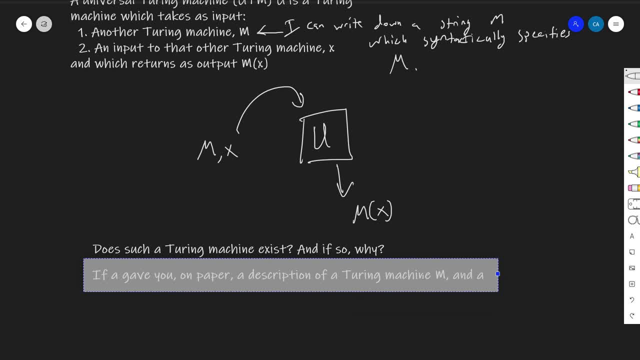 and a string and an input to that Turing machine and a string X you could, using a pencil and some time and maybe going back and reviewing those videos that I, you know, the previous videos you could. you could on paper 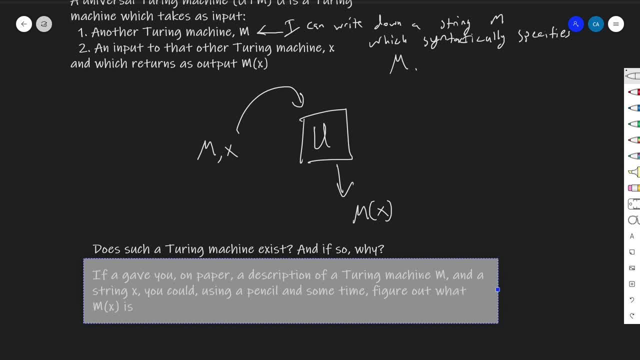 figure out what M of X is. So you could compute M of X yourself on paper. and if I gave you the Turing machine as a string and I gave you the string input to that Turing machine, you could on paper crank it out.